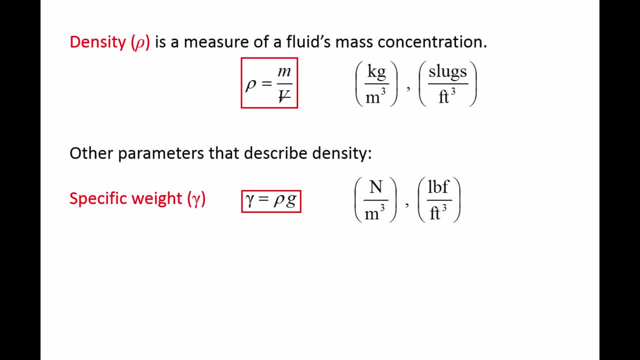 It represents the weight concentration of a fluid and its units are weight per volume. The SI units of specific weight are Newtons per cubic meter and the BG units are pounds-force divided by cubic feet. The specific gravity of a fluid is its density divided by a reference density. 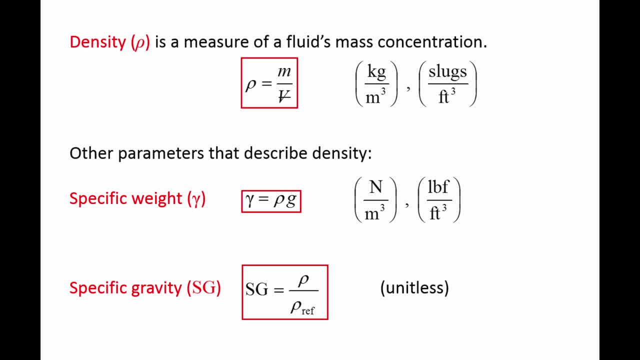 For liquids, this reference density is usually the density of water at 4 degrees Celsius, which is 1000 kg per cubic meter, And specific gravity is unitless. In general, the density of a fluid is a function of gravity. The density of a fluid is a function of gravity. 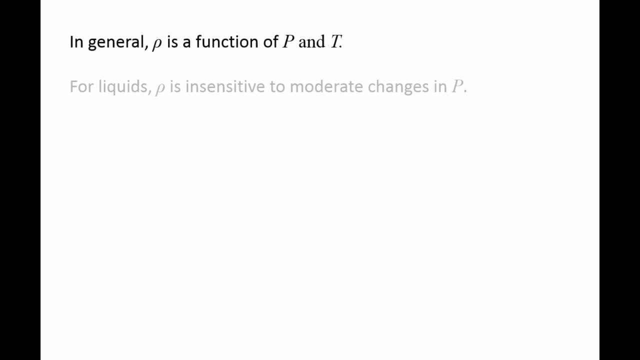 It is a function of both pressure and temperature. For liquids, density is insensitive to moderate changes in pressure. For example, the density of water at 100 kPa and 0 degrees Celsius is 999.8 kg per cubic meter. If the pressure were increased by two orders of magnitude to 10,000 kPa, the density would increase by only 0.5%. 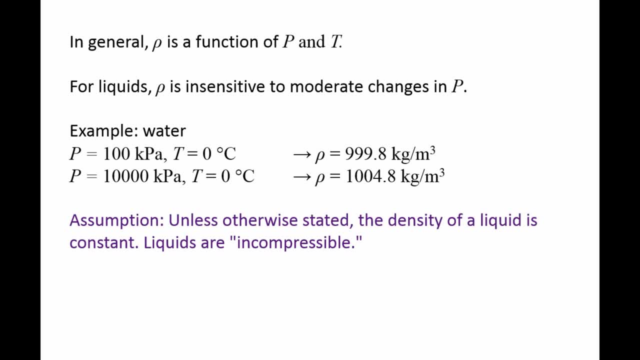 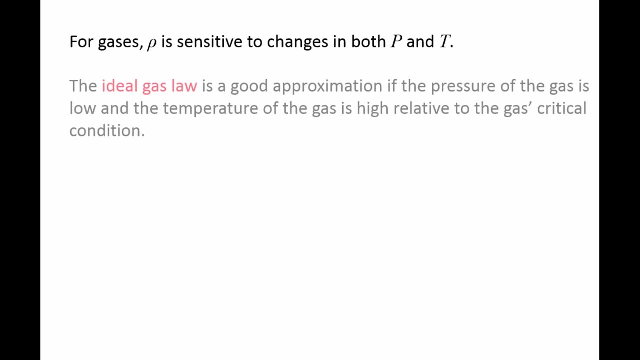 In fluid mechanics it is usually assumed that the density of a liquid is constant as it is being compressed. In other words, liquids are incompressible. The density of a gas is sensitive to changes in both pressure and temperature. Experiments show that if the pressure of a gas is low relative to its critical pressure, 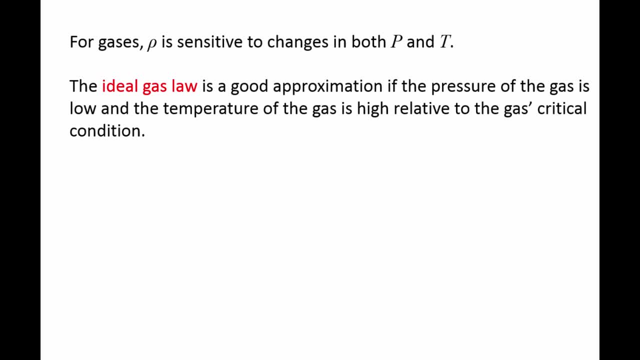 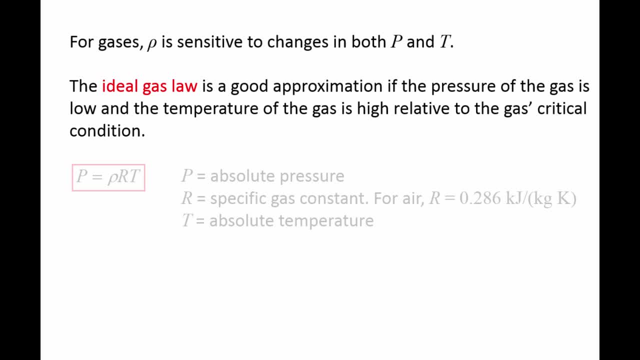 Fortunately, the ideal gas law provides a good approximation for the relationship between density, pressure and temperature. express the ideal gas law, The form that is most useful for fluid mechanics, states that the pressure of a gas is equal to its density times its specific gas constant R times the temperature.